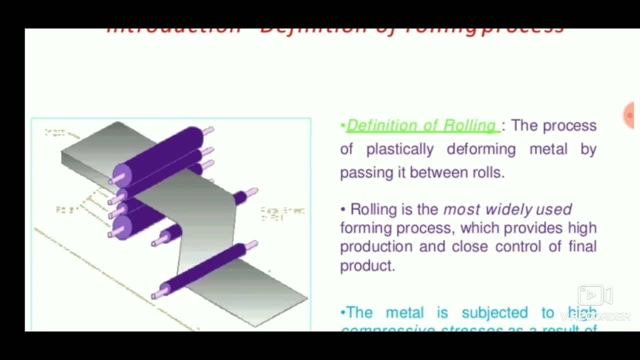 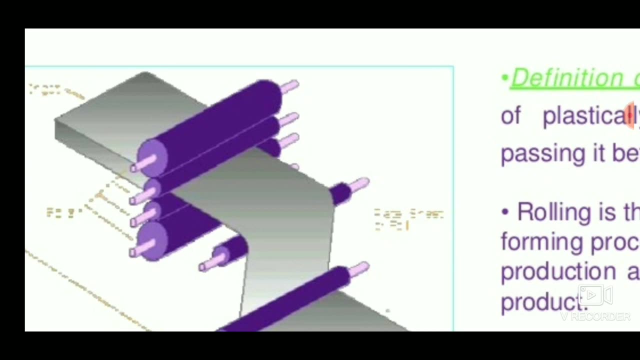 into this video. so definition of rolling is that it's the process of plastically deforming the metal by passing it between the rolls. the rolls are rotating continuously in a direction by applying the compressive force on the cast metal. so while a block of metal is applied before the 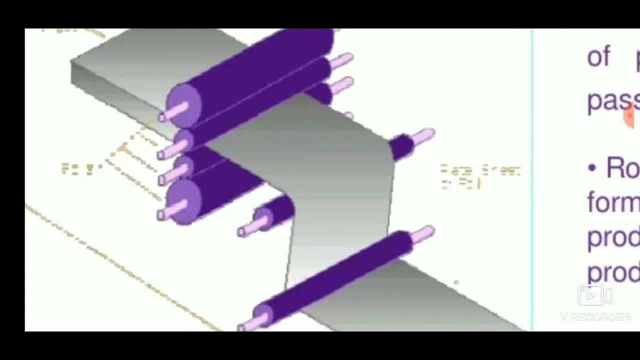 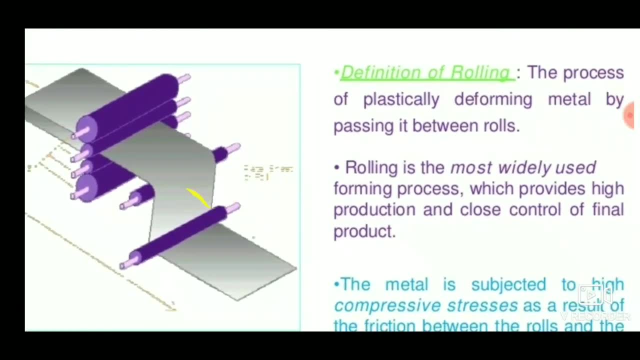 uh play appearing into the roll. after that it turns into a fine sheet. different rollers are used. let's see what are the rollers are used in this process. so rolling is the most widely used farming process, which provides the best quality of the rolling process. so let's see what are the rollers are used in this process. so rolling is the most widely used farming process, which. 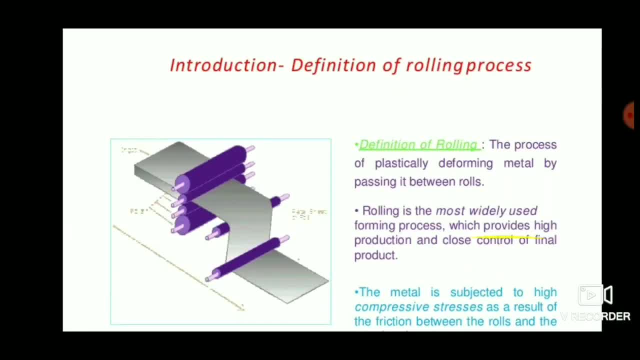 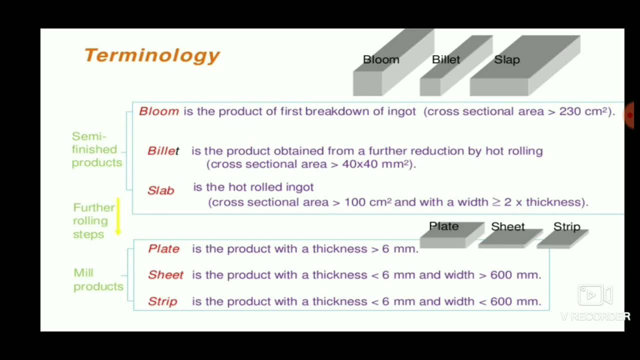 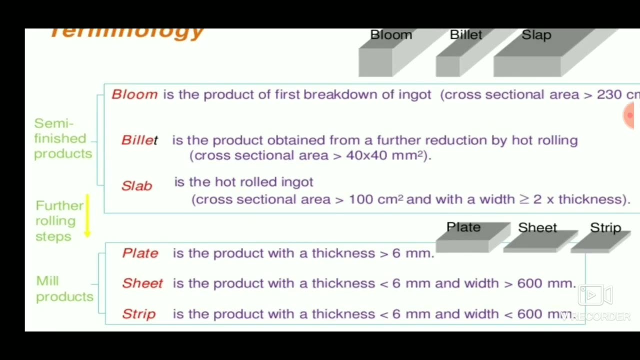 provides high production and close control of the final product. so the sheets are formed using the materials, that is, the raw material, such as bloom, billet slab, etc. so what the bloom means is a product of the first breakdown of the ingot. the cast metal is turned into an ingot. 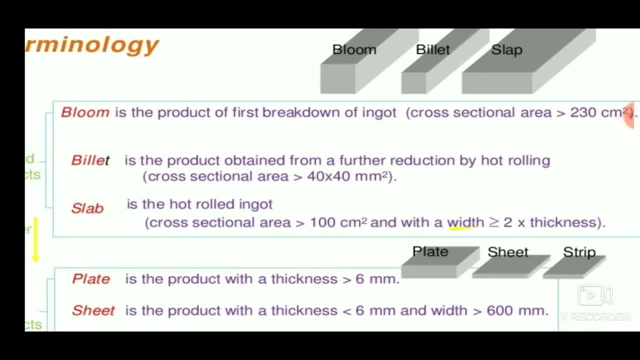 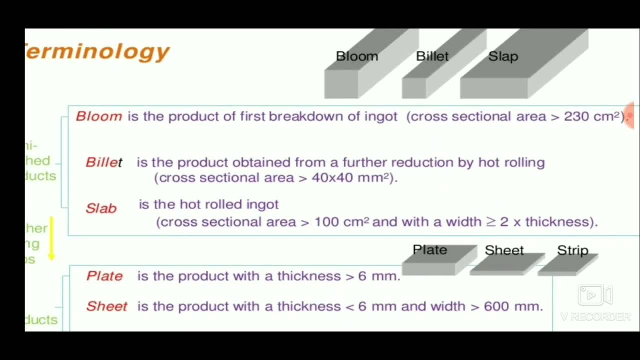 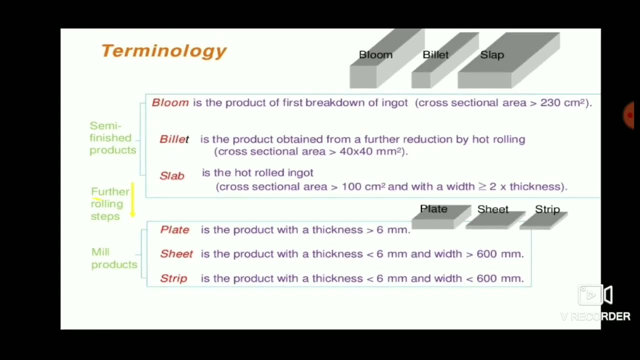 the ingot is broken down, then that this is the bloom. it is of 230 centimeter square and it is a subsystem of bloom and slab. it is a hot rolled ingot. and then it is. uh, the products appeared are plate sheet and strip of various thickness, so generally two types of rolling. 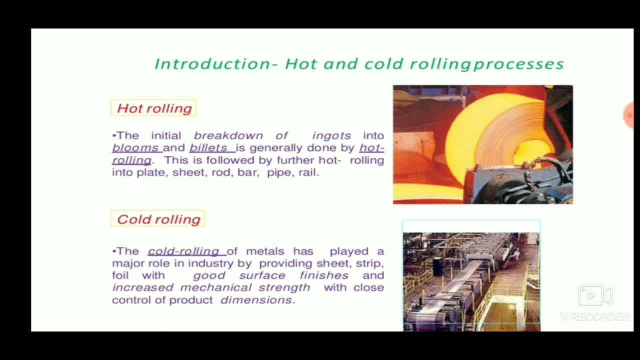 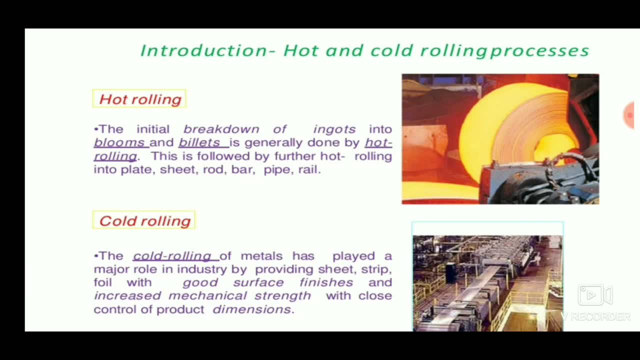 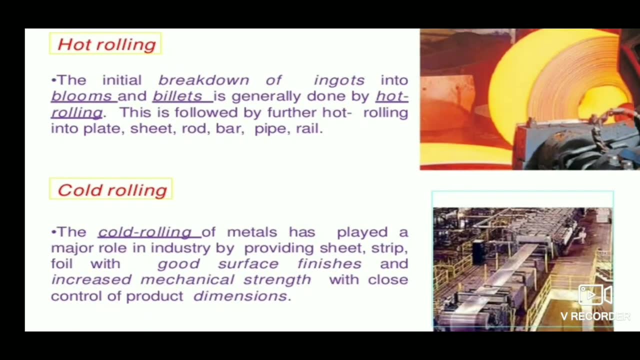 so hot rolling is the initial breakdown of ingots into blooms and billets. during this process hot rolling is used, that is, heat applied and ingots are taken out. while cold rolling the sheets plates are uh produced with good surface finish. that is called cold rolling, so generally different. 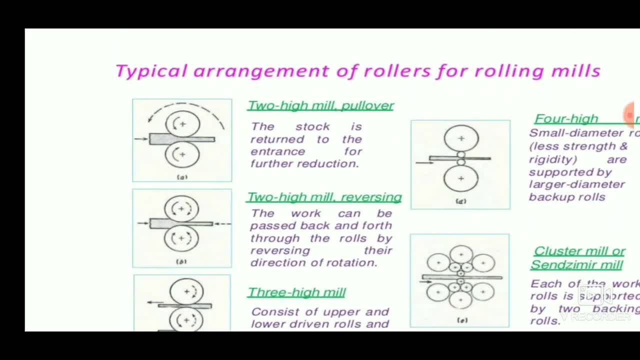 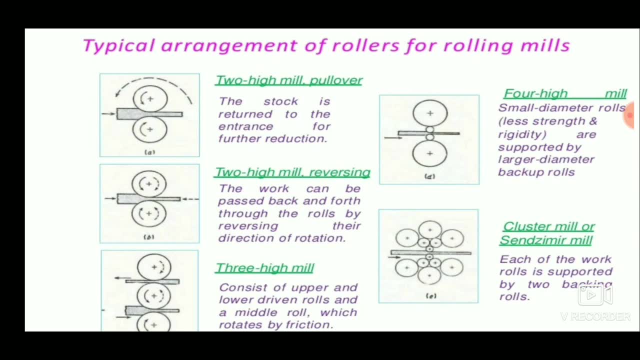 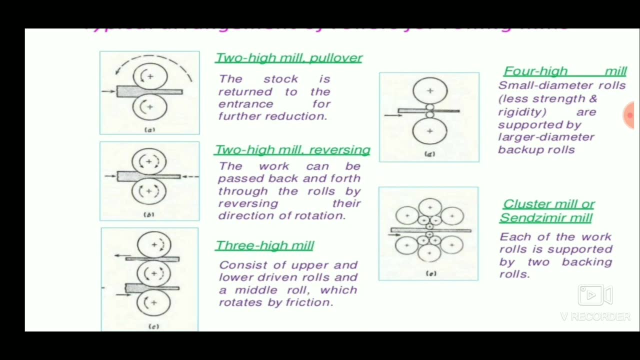 wheels and directions are applied in the rolling mills, so there are different types, such as two high mill and pullover, two high mill, reversing, three high mill used and four high mill and cluster mill are send miser mill. different mills are used for the different purposes, such as: 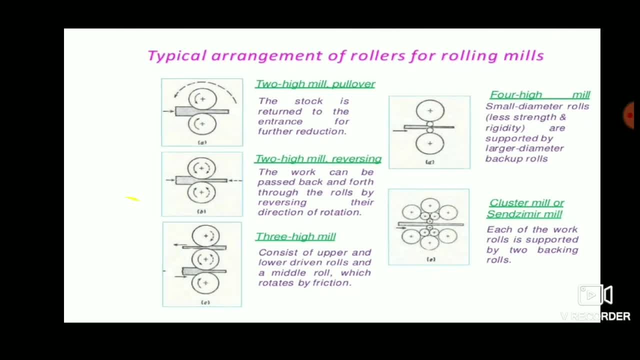 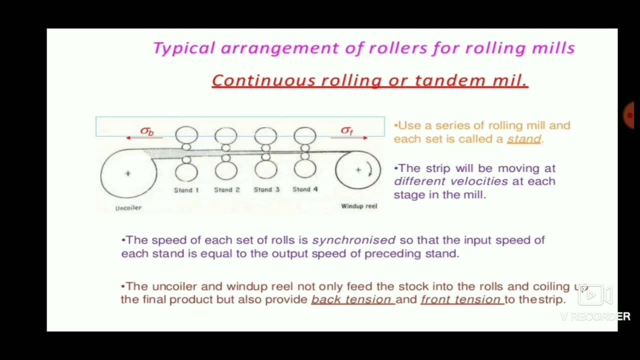 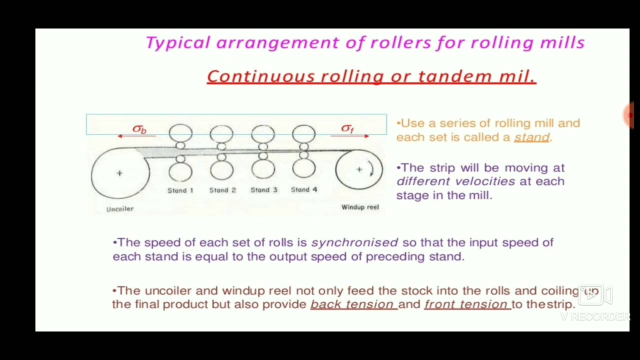 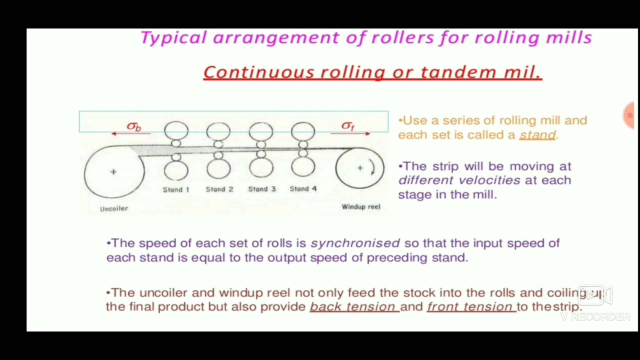 fine thickness, even grain size, etc. then continuous rolling. in this continuous rolling, different wheels of various sizes and of different compressive stresses applied to make a fine sheet in a continuous process. it uses a series of rolling mill and each set is called a stand. it is called as a stand. then the strip will be moving at different velocities at each stages in a mill to get different�um. 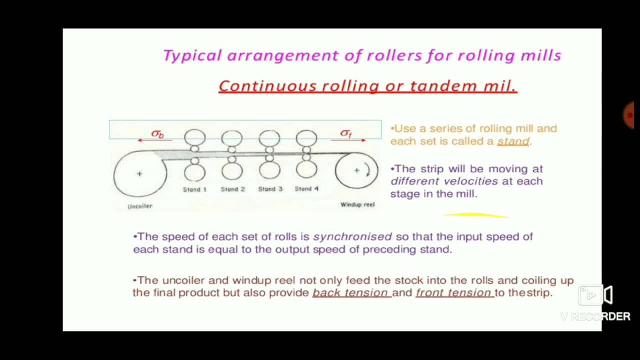 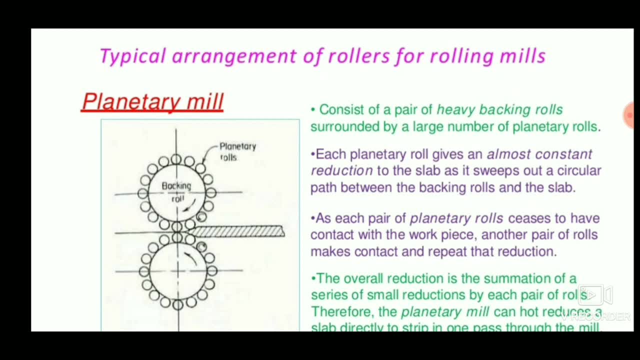 sized plates. so there is also a planetary mill. this is the planetary mill arrangement. it consists of a pair of heavy backing rolls surrounded by a large number of a planetary rolls. a small, small rollers are placed on the center roll. each planetary roll gives an almost constant reduction to the slab as 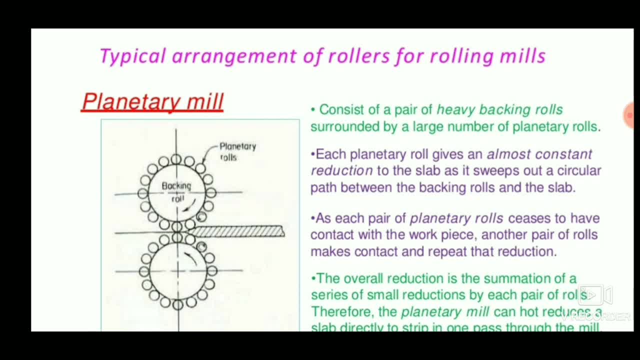 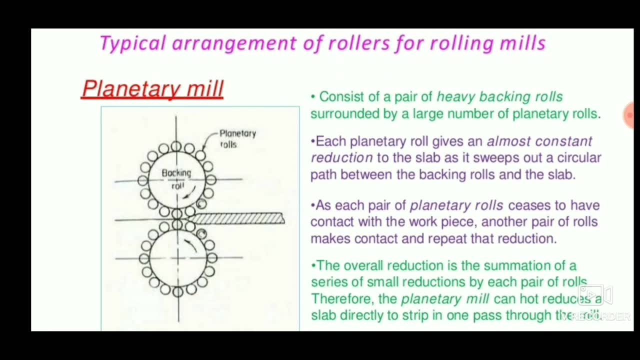 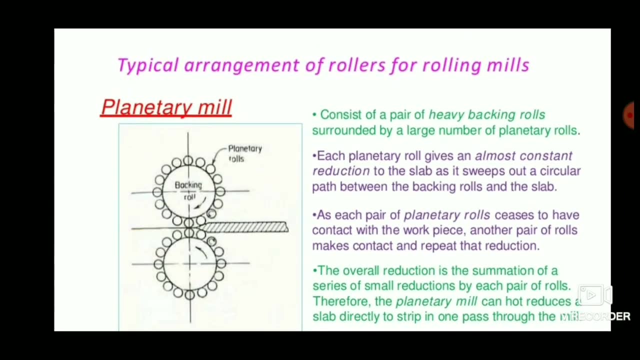 it sweeps out a circular path between the backing rolls and the slab and each planetary pair of planetary rolls ceases to have contact with the workpiece and another pair of roll makes contact with it and repeat that reduction. so this type of is used. so this is the planetary mill. that's that we have seen in. 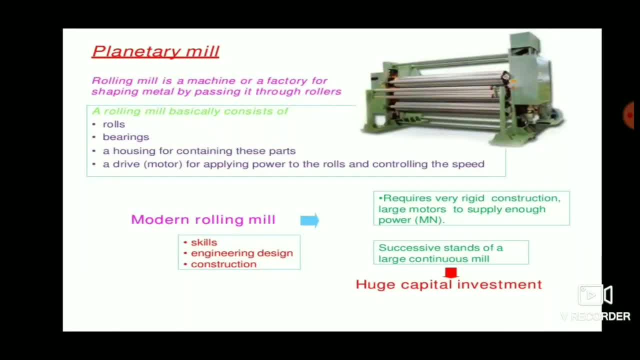 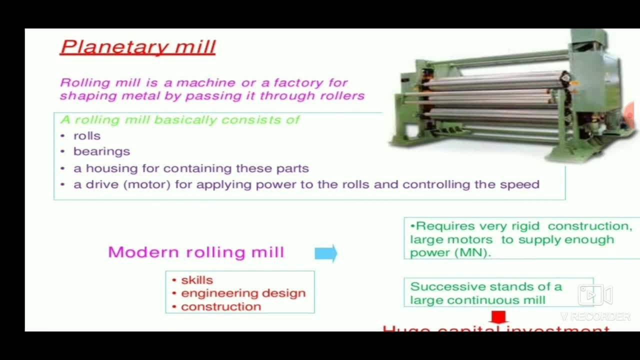 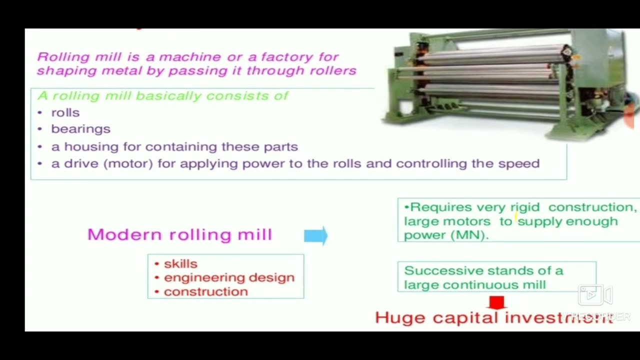 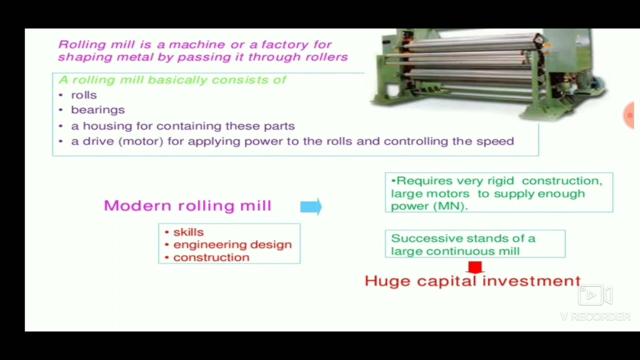 this slide. so this is the planetary mill. it is a machine or a factory for shaping the material, passing it through the rollers. the continuous small size rollers are present in this. so a rolling mill consists of a rolls, bearings, housings, a motor for actuation. then modern milling rolling mills have record a. 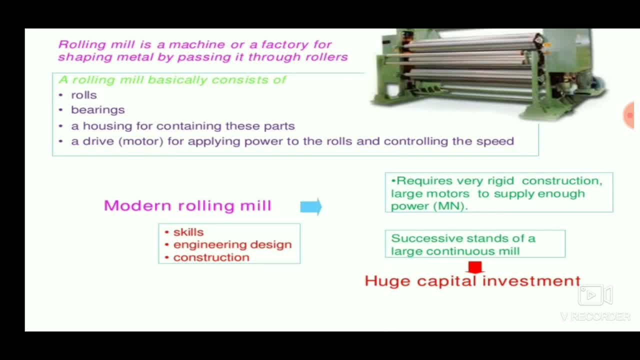 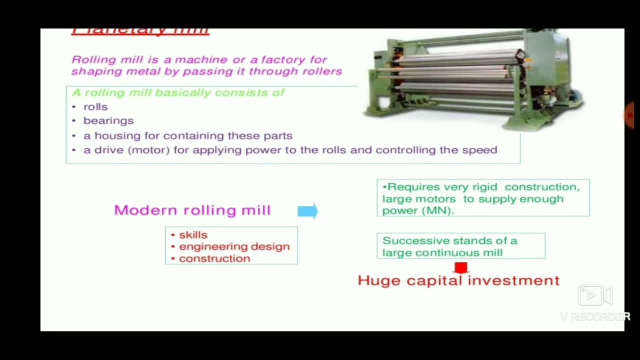 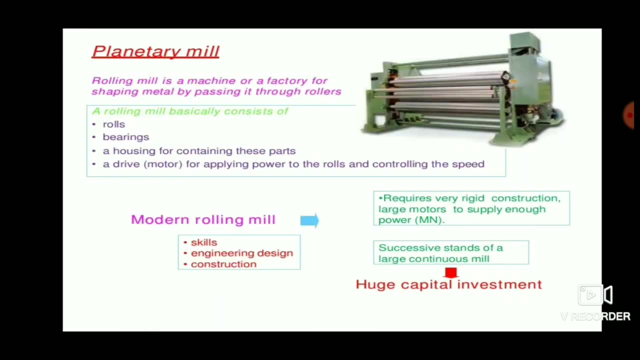 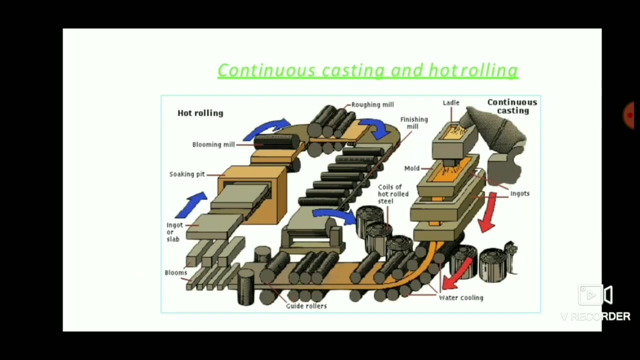 very rigid construction, large motors to supply enough power, because when you apply large compressive forces we get- we get the sheets with fine grains and with good quality. and main disadvantages of this rolling process is the huge capital investments is needed and then it is a continuous casting. yet 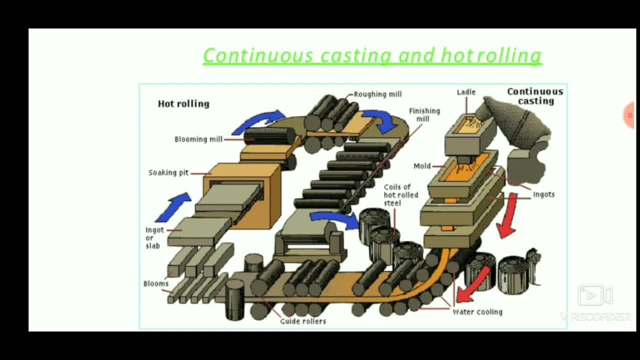 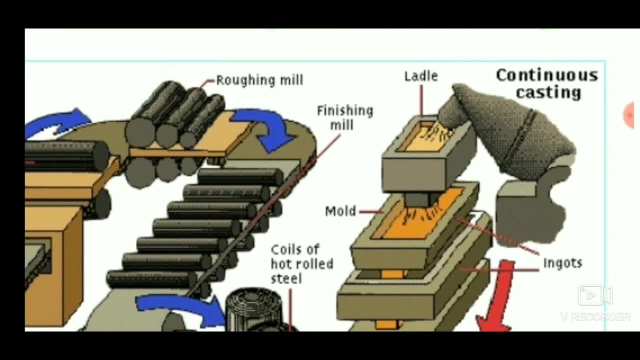 not rolling. this is the picture that shows the complete process of the hot rolling. first of all, continuous casting. the metal is molten and take it out in a ladle and placed in the mold and it's cooled over. and then it is casted on aoodle, aoodle and then it is glowed over, raising as a Steelune. molded metal from the core of the watched material needed非常的 impeniso umyusmen is needed. and then it is continued casting as a mould while rolling, then placed on the latex and then it is casted, all of these beef lightly cut into new pieces. first category, and this is the real material, the chain of the layers that consists of these beatings. we will also see it consists of: 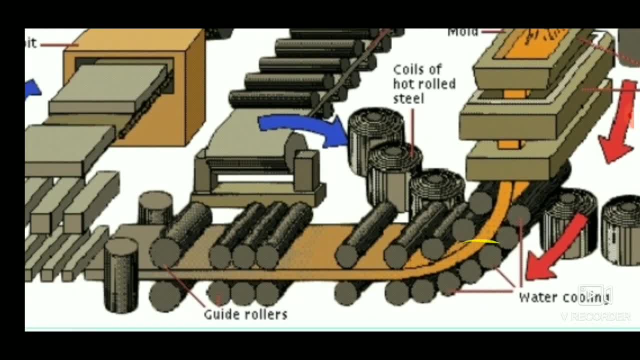 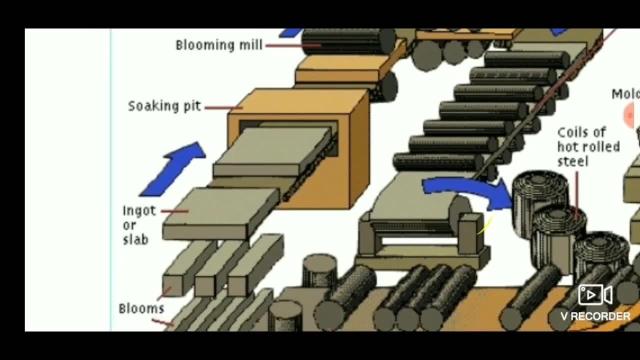 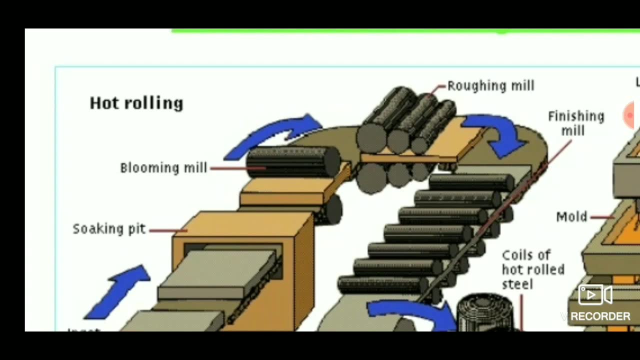 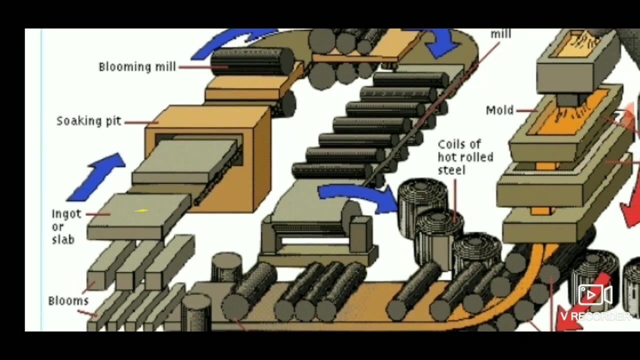 it converted into an ingot and it goes out and cut it into a blooms. the blooms are passed into the uh player- blooms are plates- are passed into the blooming mill and then it comes out in the finishing mill and then comes out as a coils of hot rolled sheet. this is what how the metal molten. 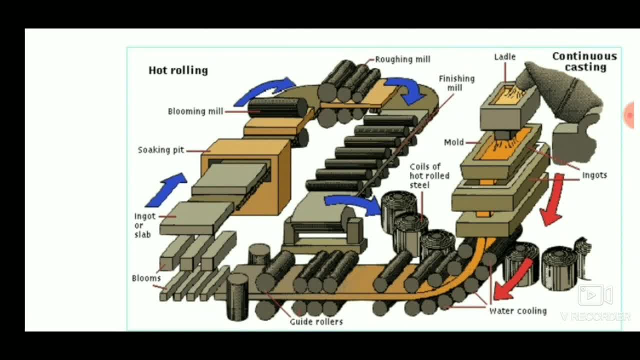 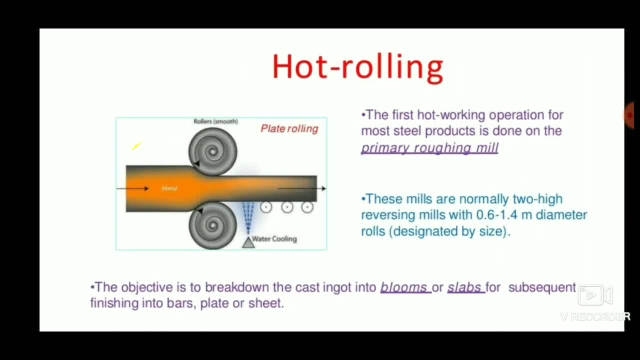 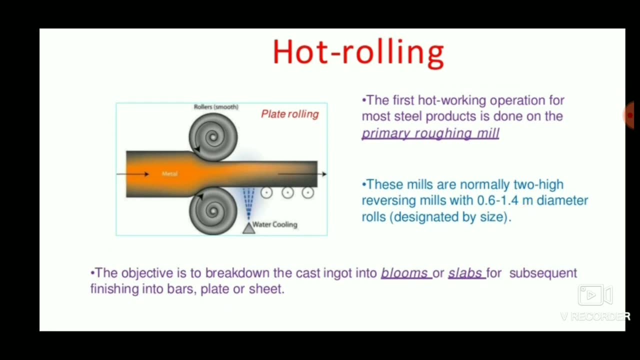 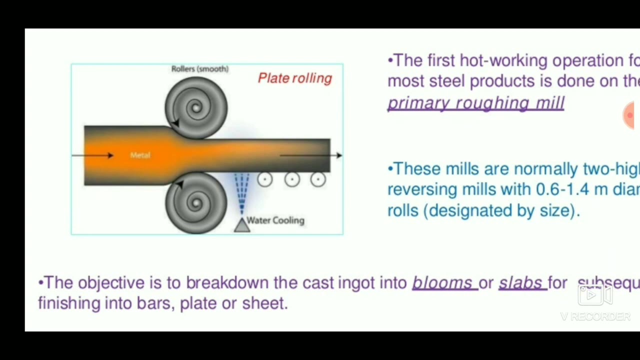 metal is turned into a sheets, blooms, slabs, etc. so during this process water cooling is applied, then hot rolling- the first hot rolling operation for most sales products- is done on the rough roughing mill. so while hot rolling, the um, a metal, that is, a cast ingot, is placed. 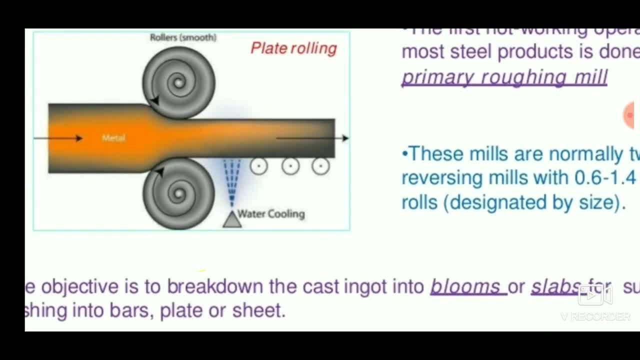 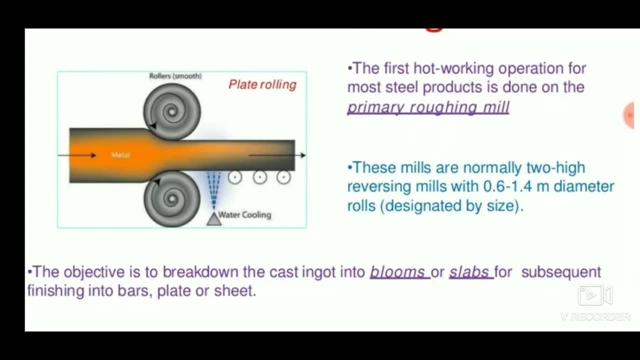 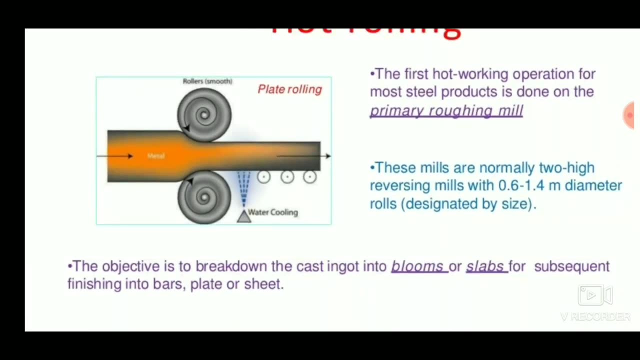 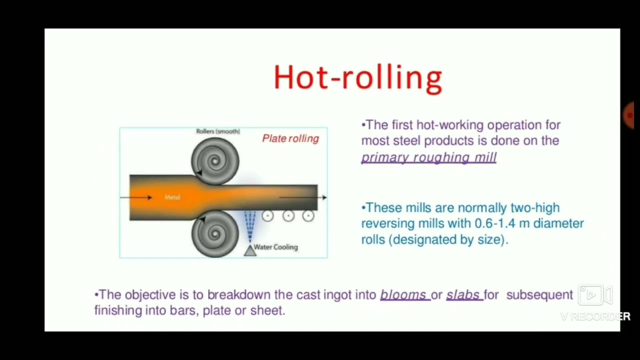 inside the two rollers. at that time water cooling is applied to make a harden of the outer surface, and these mills are normally two high reversing mills with 0.6 to 1.4 meter diameter rolls. so the main main objective is to um that, make the cast ingot into blooms or slabs making for that purpose hot. 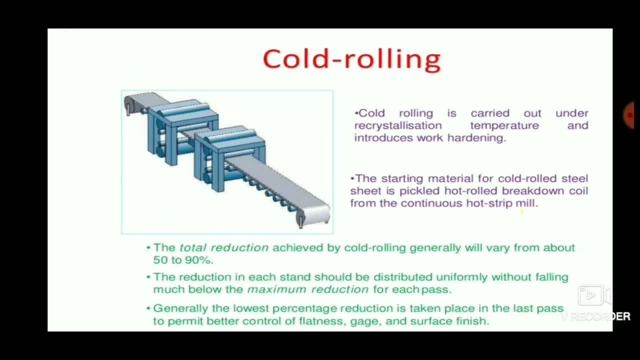 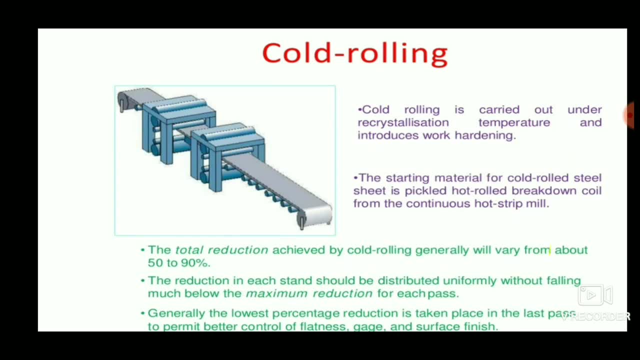 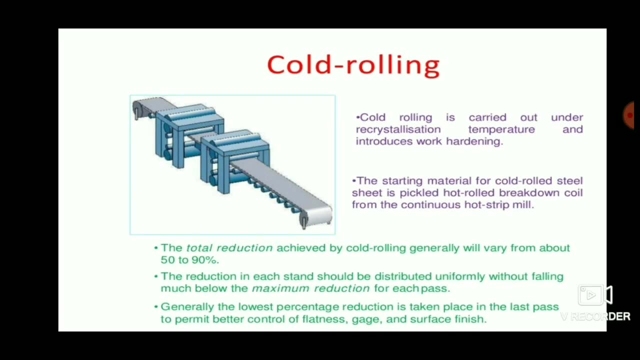 rolling is the process used then. cold rolling: it is a process. it's carried out under the recall, under station temperature, and introduces work hardening. the starting material, uh, is the uh bloom or slab, and final product is the sheet. so the total reduction achieved by the cold rolling generally, 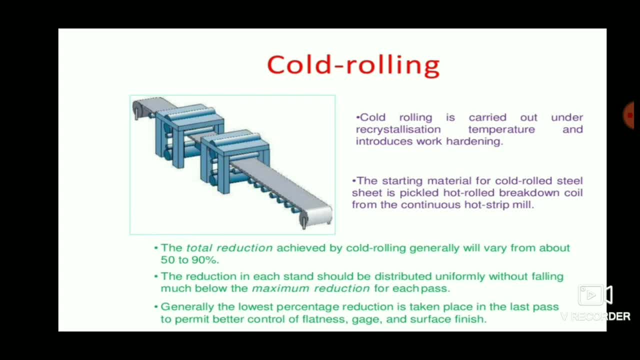 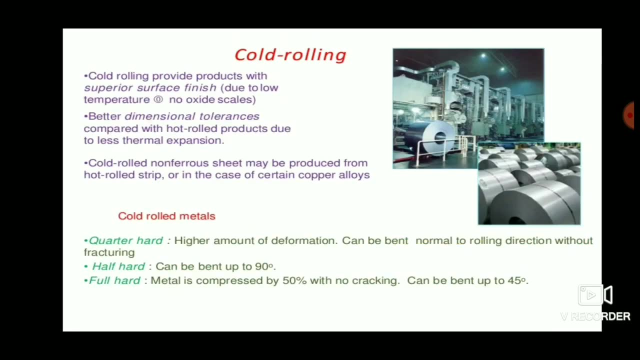 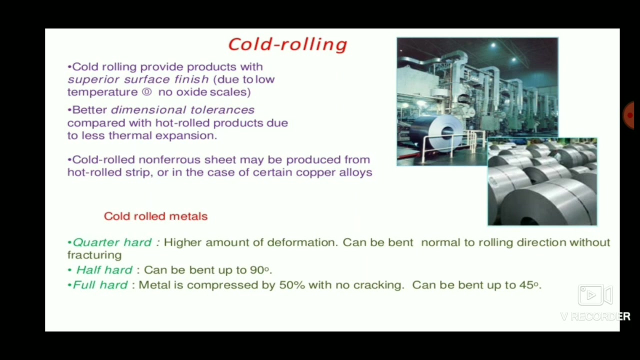 with vary about 15 to 90 percentage, and the reduction in each strand uh should be distributed uniformly without fail falling much below the maximum reduction for each pass. so the cold rolling, superior surface finish and better dimensional tolerances are achieved and it may be a good surface finish products can. 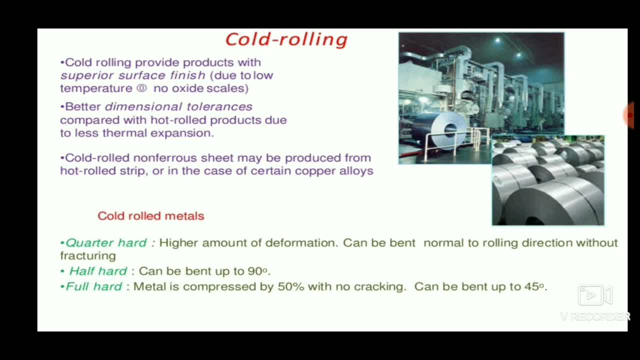 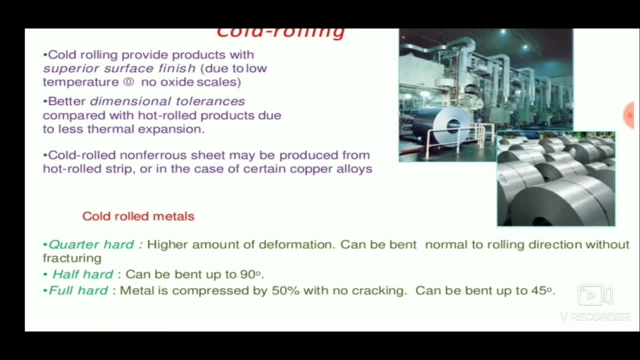 be obtained and cold round metals can be categorized into three. that is the quarter hard, that is higher amount of deformation and can be bent normal to rolling direction without fracturing. and half hot can be bent up to 90 degree. and full hard metal is compressed by 50 percentage with no cracking and can be bent up to 45 degree. these are 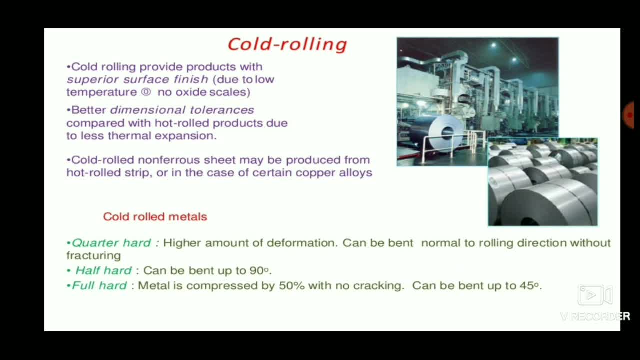 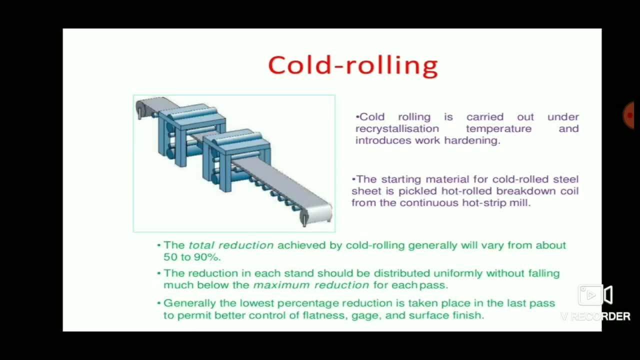 products. these are the varieties of the cold roll metals. so these are the short video about the hot rolling, cold rolling and the rolling process. so this is your video. friends, if you like this video, please click the thumbs up button and share this video to your friends to gain. 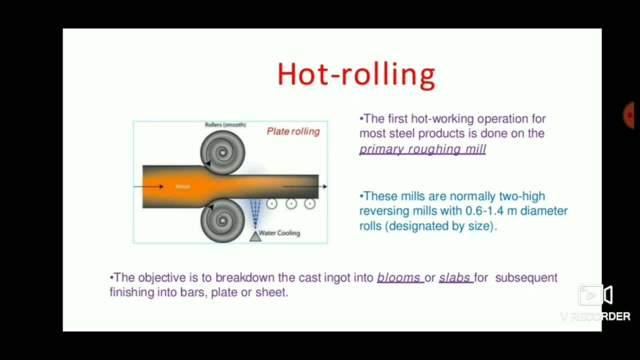 knowledge, and don't forget to subscribe this channel for more videos. so thank you for watching. 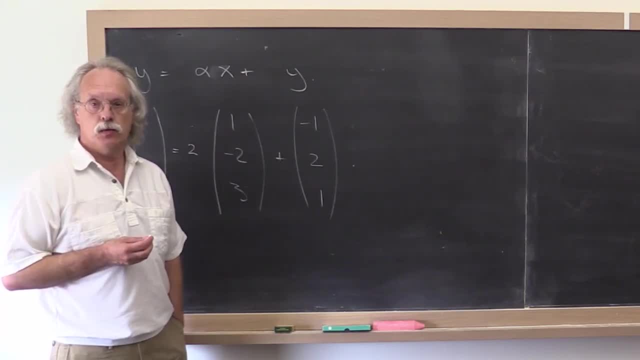 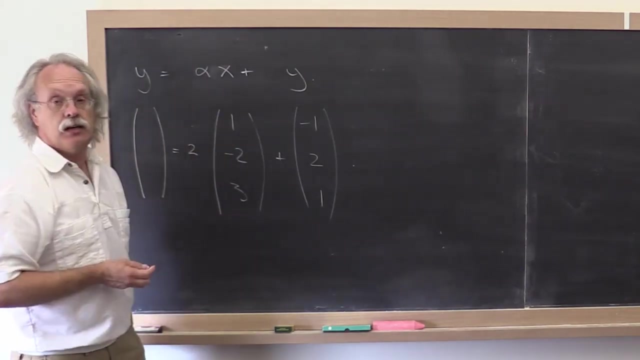 Over the years, we have noticed that a lot of the questions in week one are about these memory operations and floating-point operations, So we finally have decided to go ahead and just put a quick video about this together. So what's going on? Well, let's take the axpy operation as an example. We're doing a 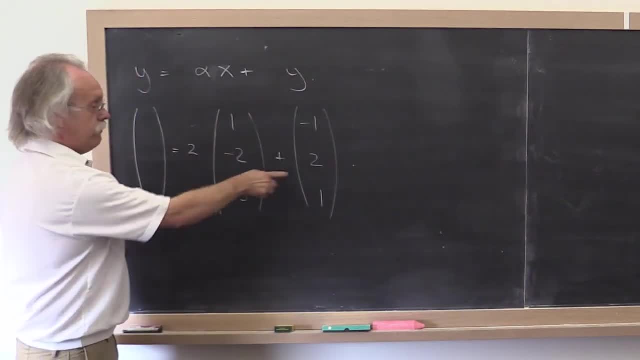 scalar times a vector plus a vector. And here we have a concrete example of vectors of size 3, where we want to do 2 times the first vector and add it to the second vector. And you've learned that that means you do this times that plus. 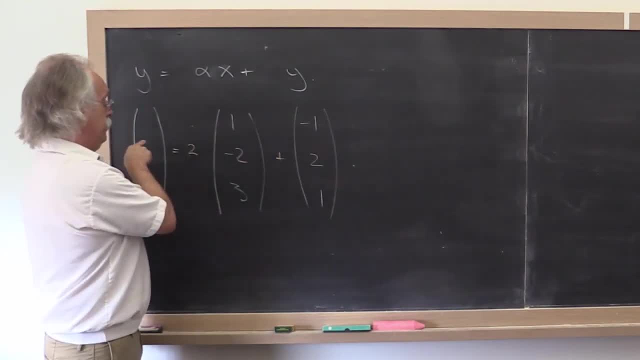 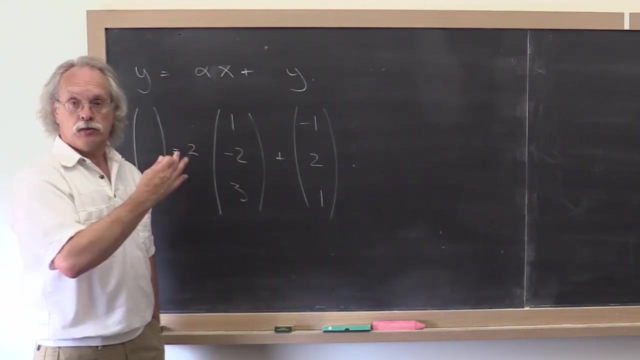 that for the first element, this times that plus that for the second element, and so forth. Now imagine that all of this data starts by being stored in the memory of a computer. In week 5, we have an enrichment that talks a little bit about. 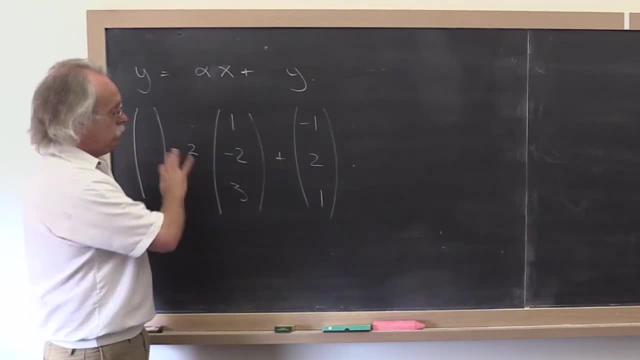 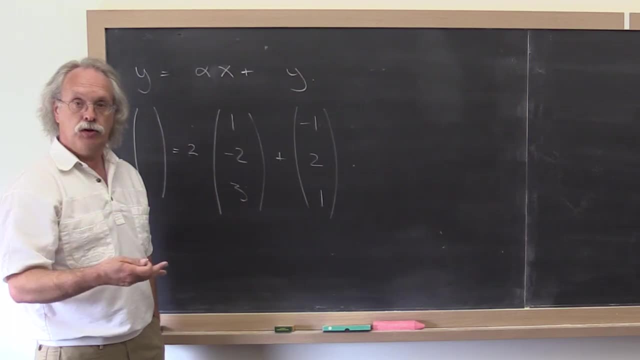 the hierarchy of memories, But for the moment just assume they're in the main memory. And the other thing you need to know is that in order for a processor to compute, data must be brought into registers, And there are only a few registers, So let's give a. 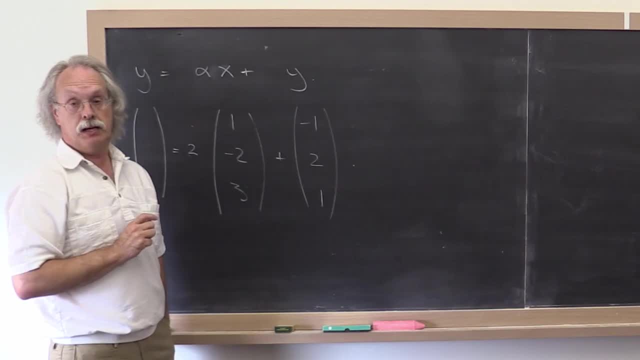 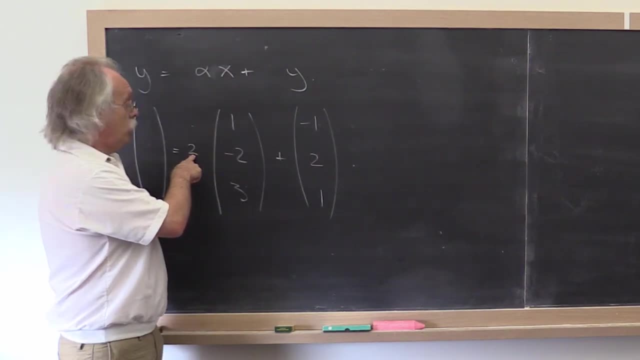 very simple explanation. This data is in main memory. We have these registers and we notice that the number 2 here gets reused many times. So what we can do is we can take 2 and we can load it into a register and keep it there during the